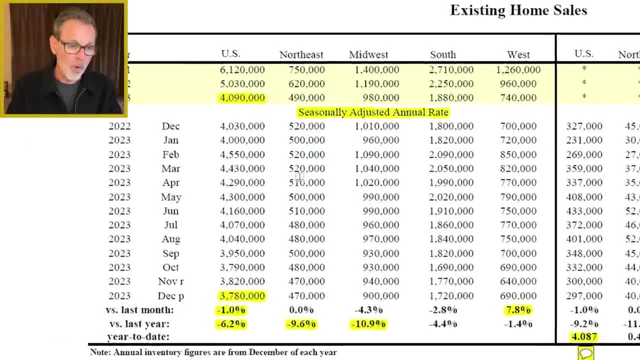 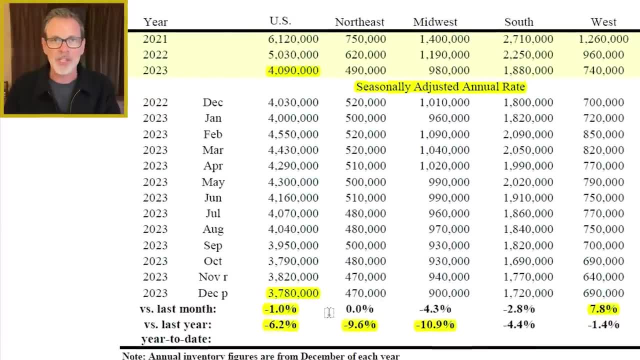 for each of these major regions. So for the US as a whole there was 3.78 million. That was the sales base. Again, the seasonally adjusted annualized sale pays for December was just under 3.8 million. That's a decrease of 1% compared to November and down 6.2%. 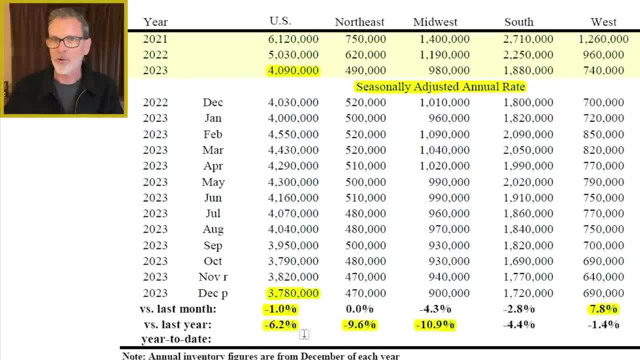 year-over-year. Now again, every housing market's different right. Your city can vary greatly depending on what's happening in the nation, And, of course, each of the regions can vary as well. As you can see right here, the Northeast was flat on a month-to-month basis, whereas the West surged by 7.8%. That was December sales pace compared to November. On a year-over-year basis, all four US regions decreased And actually we saw the biggest declines in the Northeast, down by 9.6%, and the Midwest fell by. 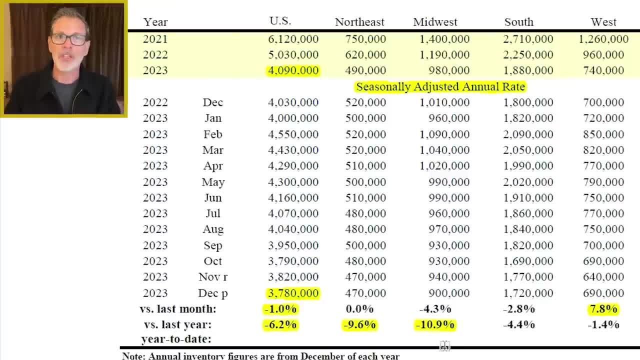 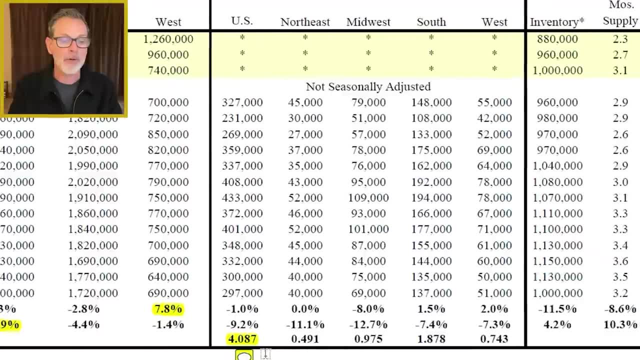 about 11%. Now, when accounting for the fact regarding the total number of actual home sales for the entire year of 2023, it came in at 4,087,000.. That was down 9.2% compared to the year And, in fact, the biggest declines were actually in the Northeast, down by 11.1%. 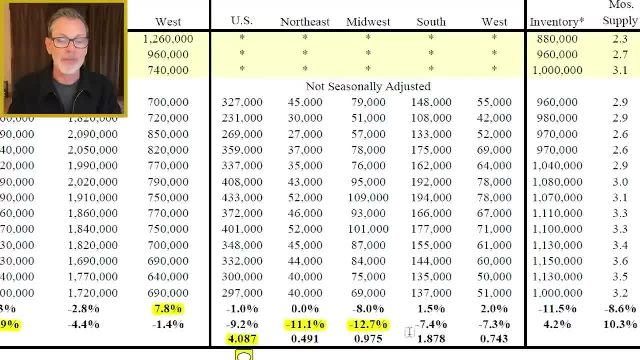 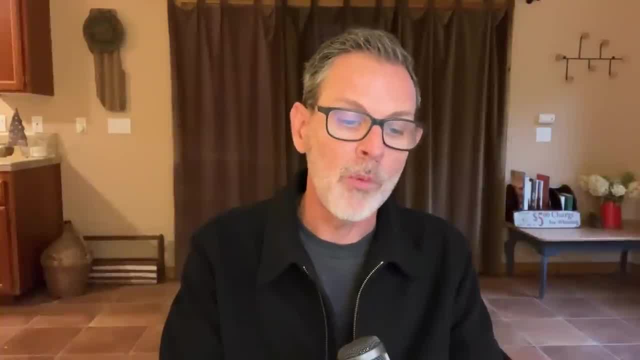 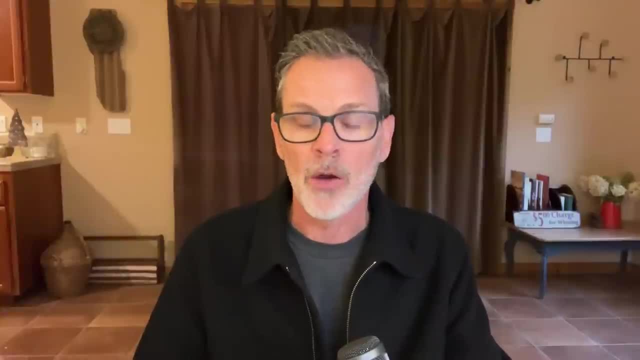 and down by 9.2%: 12.7 percent in the midwest, whereas the south and the west decreased by around seven percent. so, now that we know that, the total number of home sales- this is existing home sales for single family houses, condos, co-ops and a townhouses, townhouses, i should say so- just under 4.1 million, as you can. 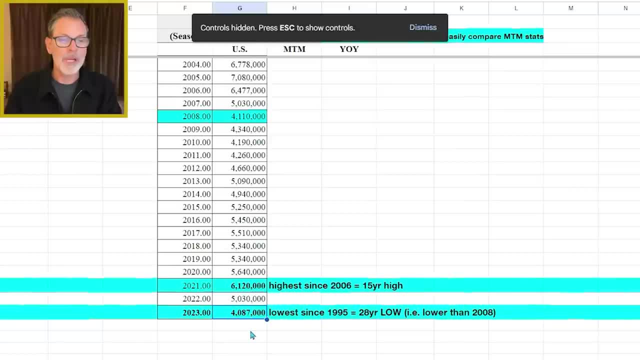 see right here, based on my nerdy excel formula here. so by my own analysis of nars data here, at 4.087 million, that's the lowest levels since 1995.. in other words, a 28-year low regarding closed home sales in the us for the whole year of 2023, which is quite remarkable because that is. 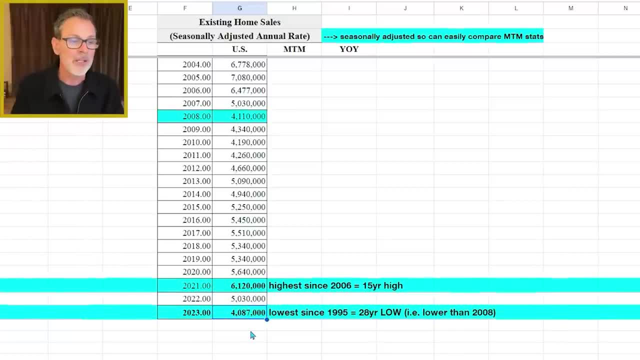 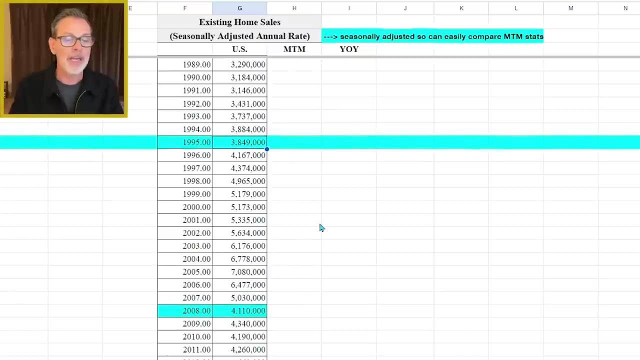 actually less than what we saw back in 2008. so, for example, 2008 it was about 4 million 110 000. now we're under 4.1, 1 million again, the lowest number of close home sales for the entire year since 1995. when at that. 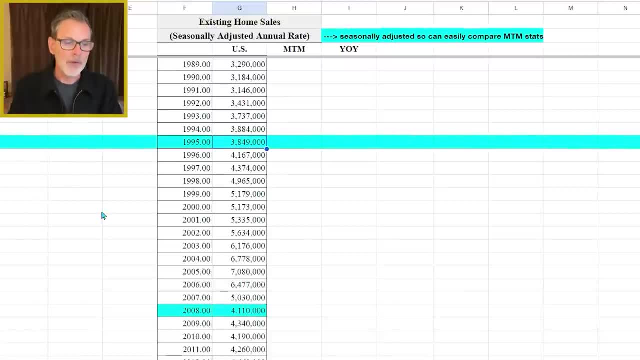 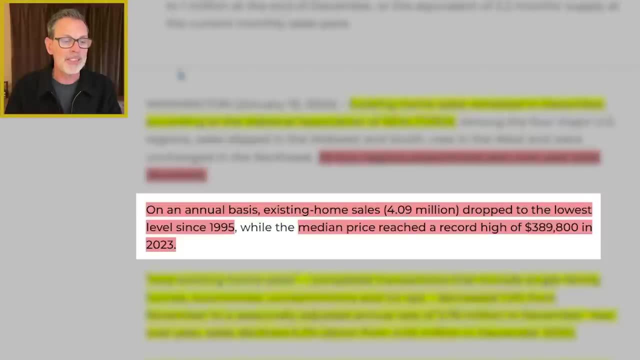 time there was about 3.85 million. in regards to that, that's exactly what the national association realtors had to say as well, because on an annual basis, existing home sales decrease to the lowest levels since 1995.. they also mentioned that the meeting sold price reached an all-time record high. of just under 390 000. how they came up with that figure, though, was the median sole price for the entire year of 2023, and compare that to 2022.. a small gain from 2022, which was the previous all-time record high, and now it's at nearly 390 000.. i'll provide an additional analysis regarding 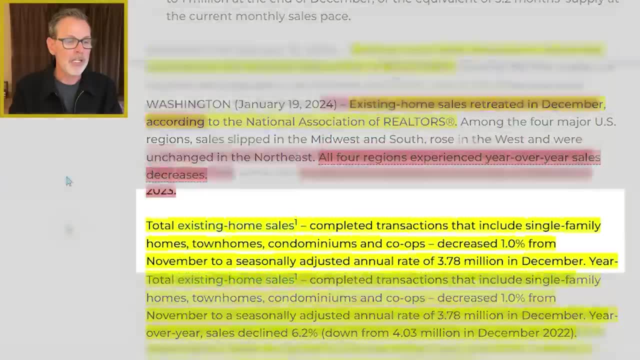 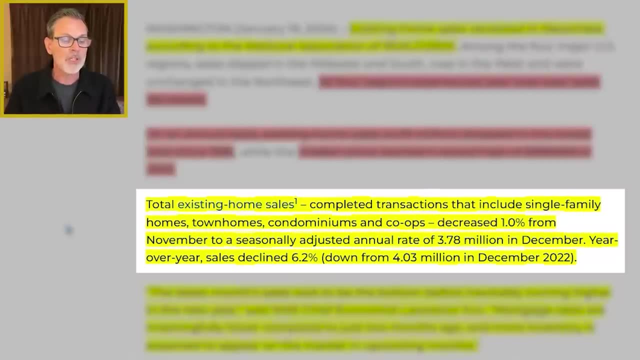 home sold prices here in just a little bit regarding existing home sales, which are completed for a very small amount of time. it's not like we're doing the houses that we've looked at here already, which is the things that we've been talking about in the in the first two videos. 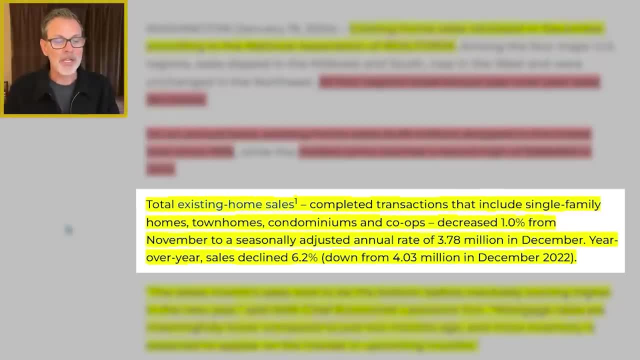 over and, over and over again, which is 2 million of sales by the end of this year and the first round of sales over the second week of this year as well. so you would be able to see an increase. but what i know that a lot of people are not going to do is kind of just weight and do a lot of 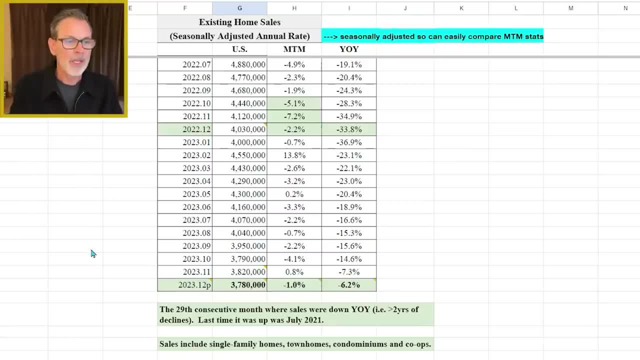 extra work on the home or have to maintain the home as they are before and after the beginning of the year in a bluegrass area because the demand is probably going to be quite negative because these date and also the seasonally adjusted, analyzed pace of close home sales of existing houses on a 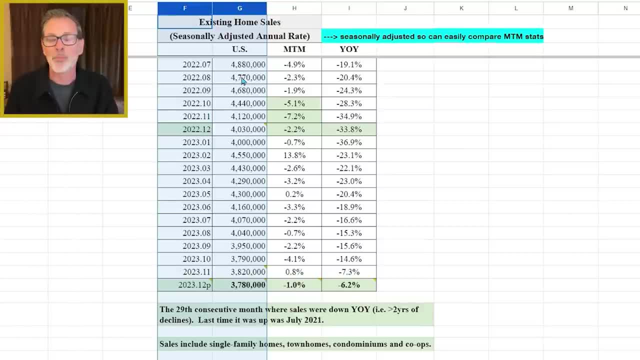 national level. that is actually the only data i pulled from the national association of realtors website. everything else is based on my own analysis here. so again, this december it came at 3.78 million. that was actually below the forecast, which was at 3.82 million. also that current sales. 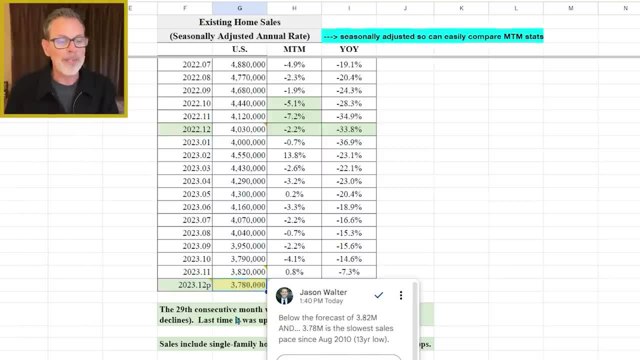 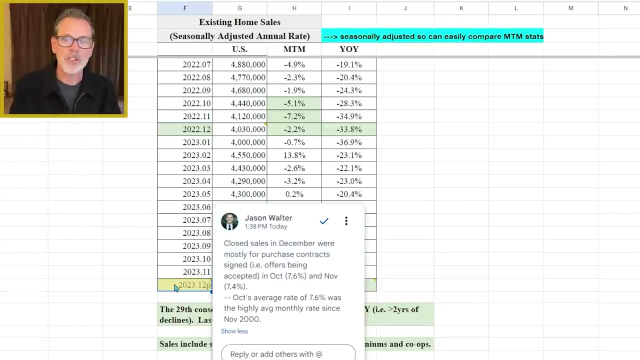 pace, or just a december sales pace of 3.78 million, is actually the slowest sales pace going back to august of 2010.. in other words, the pace of close home sales in december was nearly eight, or actually not nearly- was a 13 year low. now something to keep in mind as well when looking at close home sales. 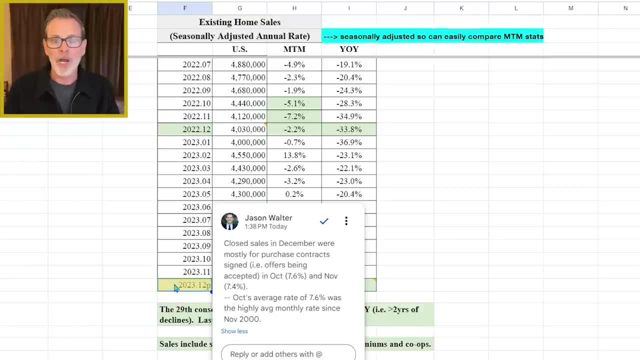 to 7.4% in November. Now keep in mind, though, the pace or not the pace, the rate back in October at 7.62% was actually the highest monthly rate since November of 2000.. So, of course, having said, 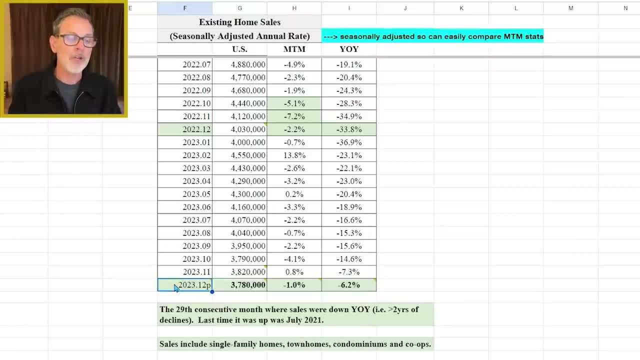 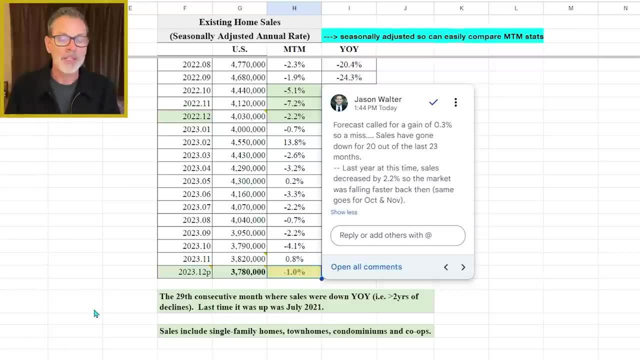 that it makes sense that home sales remained very, very low in December. Also, like I mentioned previously, sales actually decreased compared to November as well, down by 1%. The forecast, by the way, was calling for a gain of 0.3%, So it came in below the streets forecast here. 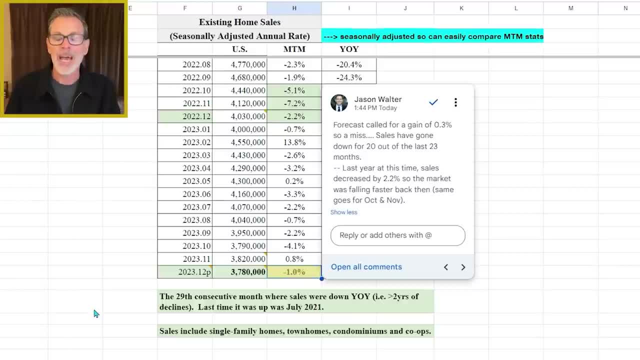 Home sales have also gone down for 20 out of the past 23 months. How wild is that? There's basically only three months of home sales that have gone down, So that's a lot of money. So in which home sales were going up but down in 20 of the past 23 months? One thing to keep in mind. 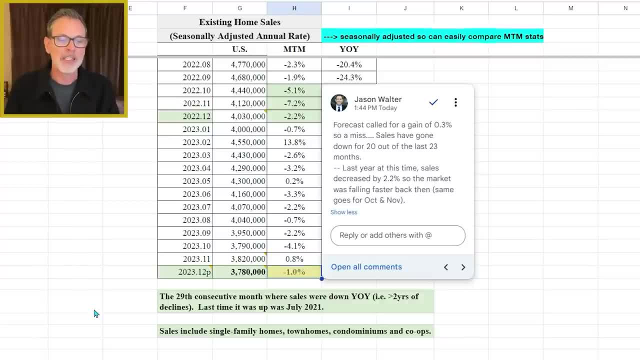 though I mentioned this over the past several months, is that last year, this time, sales decreased much greater compared to this year. So, for example, this December down by 1%, but in December of 2022, it fell, or home sales fell by 2.2%. 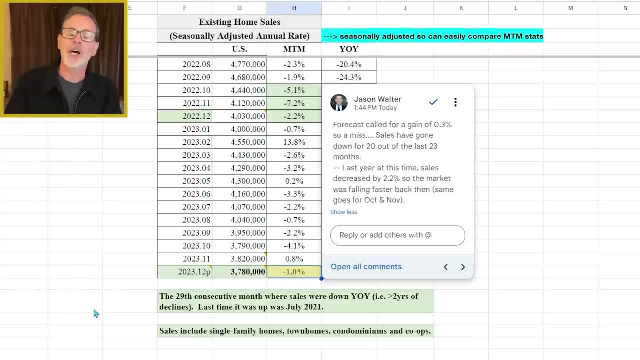 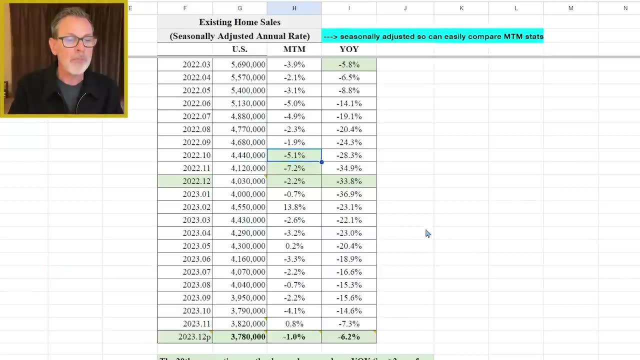 So, therefore, the market was falling much faster in 2022 compared to the last half of 2023.. We also can see this similar scenario here back in October and November as well. Don't take my word for it, though. Look at this. So in October of 2022, home sales decreased. 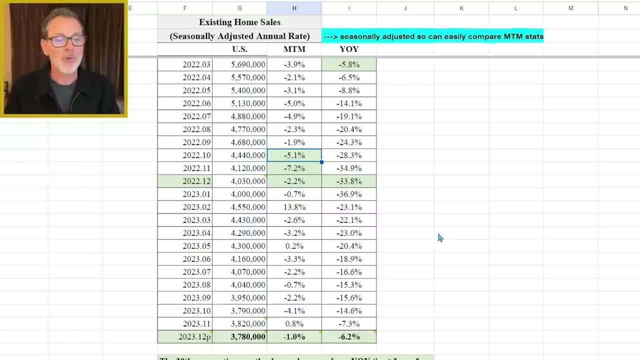 by 5.1%. That was a decrease in sales from September through October, The month-to-month change down by 5.1%, But in October of 2023, it decreased only by 4.1%. Then in November last year- or 2022, I should say- it decreased by 7.2% in one single month. 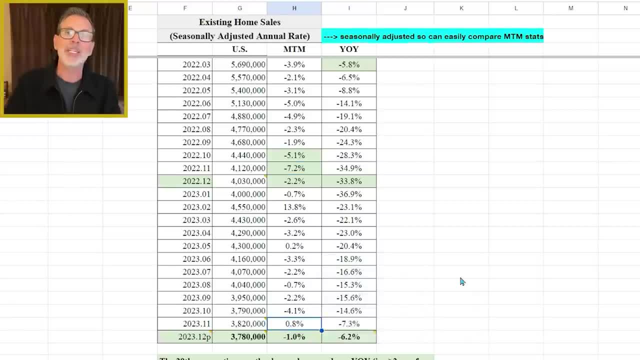 Whereas November of 2023, it actually increased by 0.8% And also last December, it fell by 2.2%, This last December, December of 2023, it fell by 1%, So overall home sales were falling much. 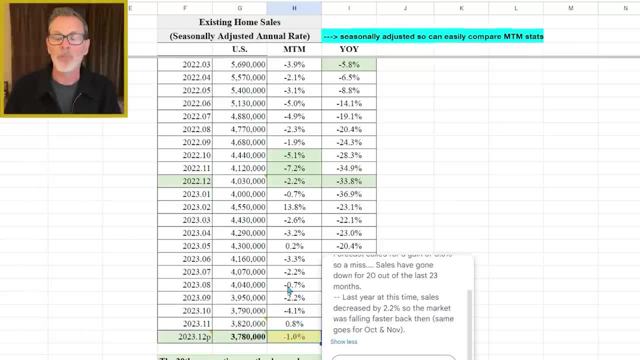 faster in the last half of 2022 compared to the last half of 2023. And that's actually one of the reasons why the year-over-year changes are not as bad as what they were back in 2022. So, for example, in December of 2023, compared to December of 2022,. 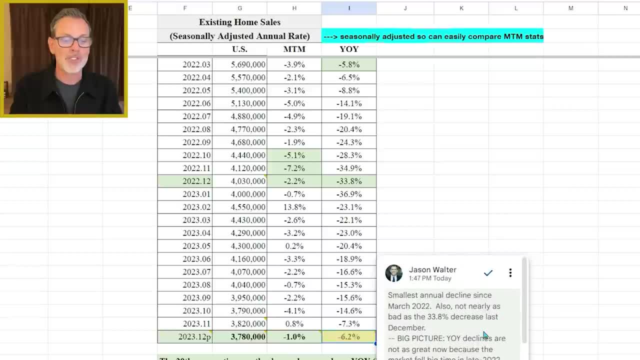 the year-over-year change fell by 6.2%. That actually was the smallest annual decrease since March of 2022. So, for example, back in March of 2022, it fell only by 5.8%, Whereas this year it decreased by 6.2%, which is not as bad as December of 2022,. 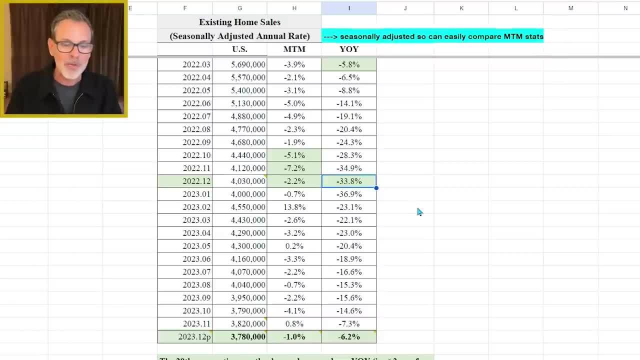 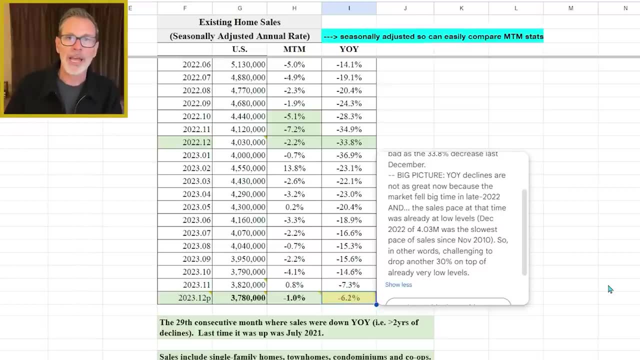 where home sales tanked by 33.8%. So, as a note right here, big picture, the year-over-year declines are not as great as what they were back in 2022, or last half of 2022, compared to last half of 2023.. And this of 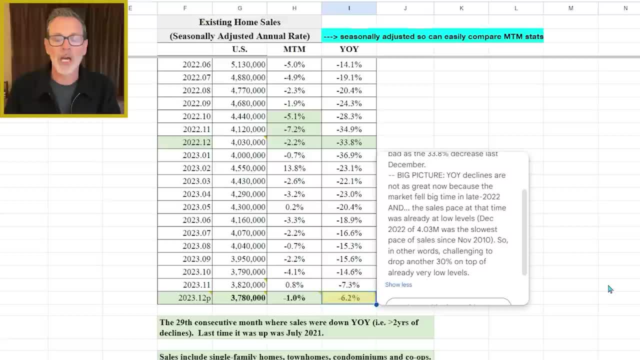 course is because the market was falling big time in 2022. And the sales pace in December of 2022 were already at very low levels. In fact, back in December of 2022, the sales pace back then was 4,030,000 closed home sales. That actually was the slowest pace. 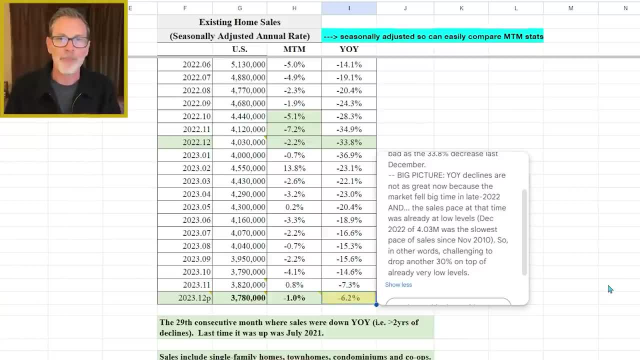 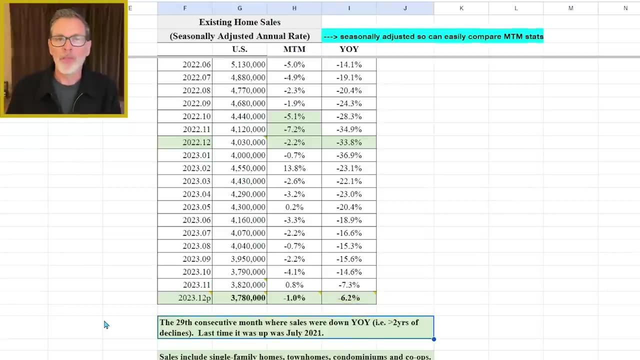 since November of 2010.. So, in other words, here it's very challenging to drop another- let's just say another- 30%, given the fact that back in December of 2022, we were already at very, very low levels. One more thing I do want to add regarding this table here: 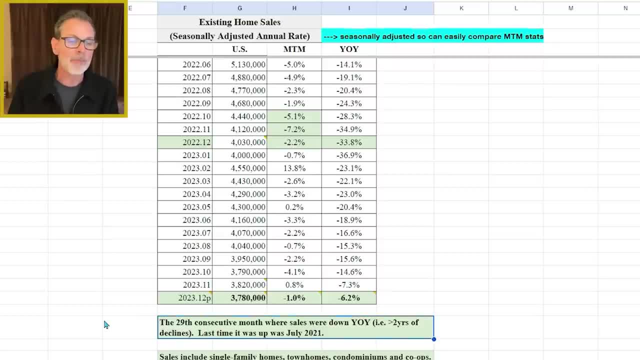 is that this marks actually the 29th consecutive months in which sales were down on a year-over-year basis. In other words, we have more than two years of declines on a year-over-year basis. The last time home sales were up was back in July of 2021.. 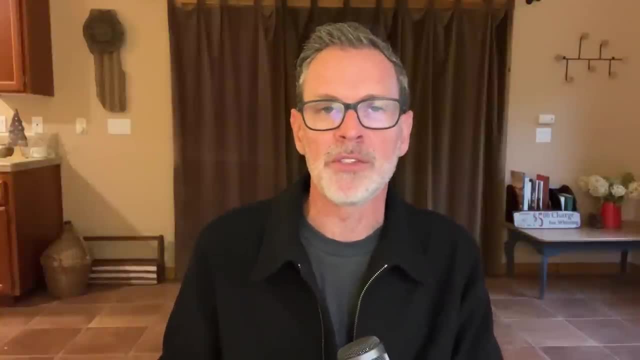 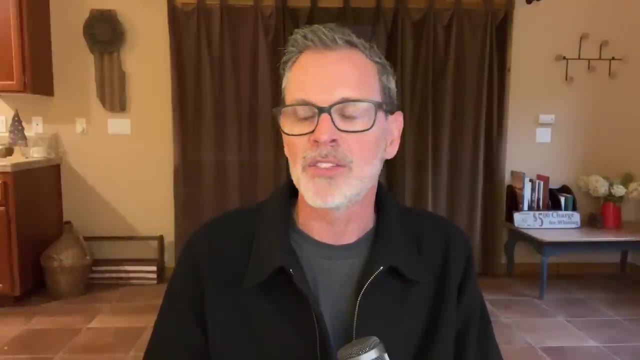 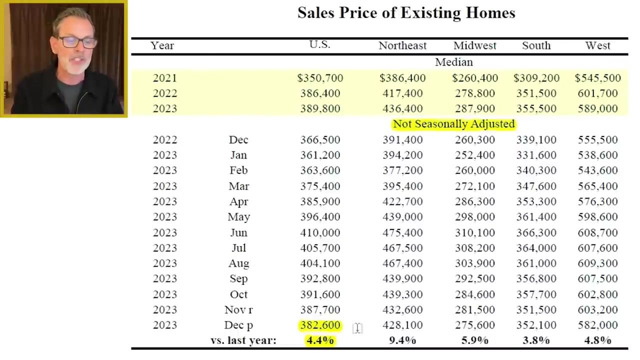 Okay, let's change gears slightly here and talk about home prices. And when I'm talking about home prices in today's video, I'm talking about the median sole price in the US, unless otherwise noted here. So overall in the US for December the median sole price- not seasonally adjusted- came. 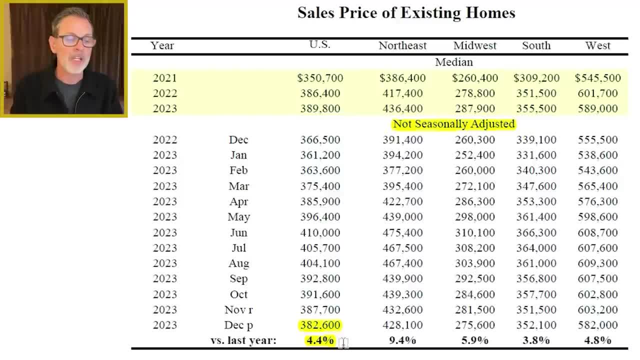 in at just under 383,000.. That was up by 4.4% compared to December of 2022.. Home prices increased the most, actually in the Northeast, increasing by 9.4% over the past 12 months. 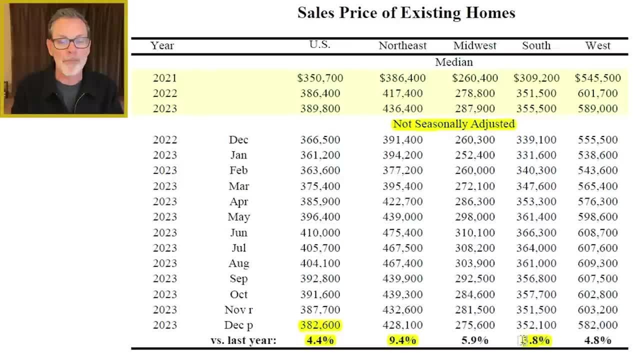 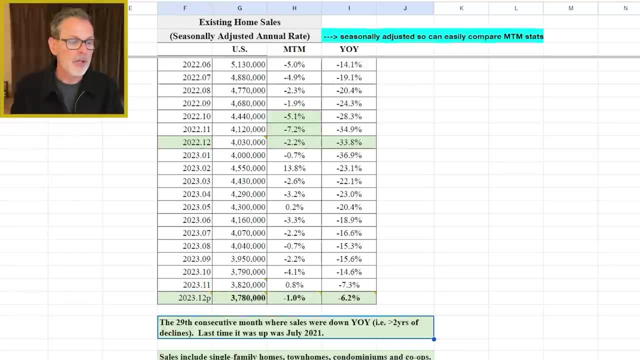 whereas the South only increased by 3.8%, The West increased by 4.8% and the Midwest increased by 6%. So that is their analysis. here Let me share my own analysis. So again for the year as a whole. 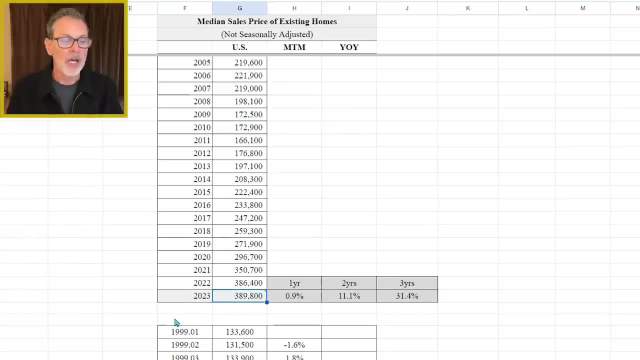 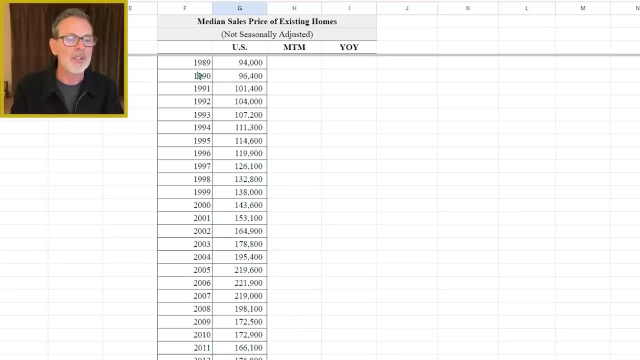 the median sole price for the entire year came in at just under 390,000, an all-time record high for data that goes back until 1989. Look at that: 1989, the median sole price was $94,000! Absolutely crazy. I know that rates were around 15% back then. 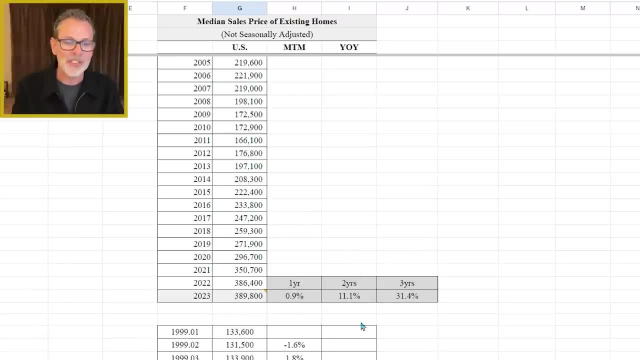 but still $94,000 compared to $390,000 right now. So, in any case, looking at the annual change in prices, the annual change only increased by 0.9%. Again, the median sole price for the entire year of 2022 compared to 2023, with a small gain of 0.9%. 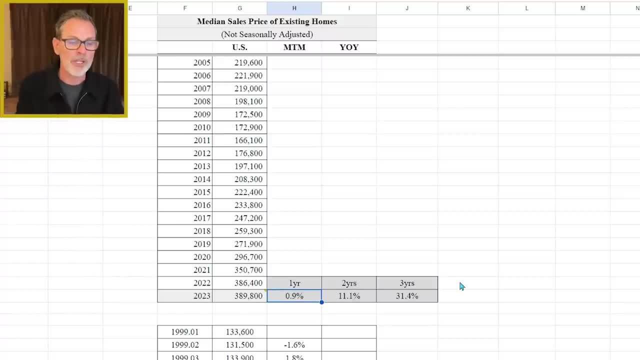 This alters the median, And here's what the median sole price has become compared to 2021.. The median sole price for the entire year of 2022: compared to 2023, a small gain of 0.98%. The median sole price for the entire year of 2022: compared to 2023, a small gain of 0.98%. 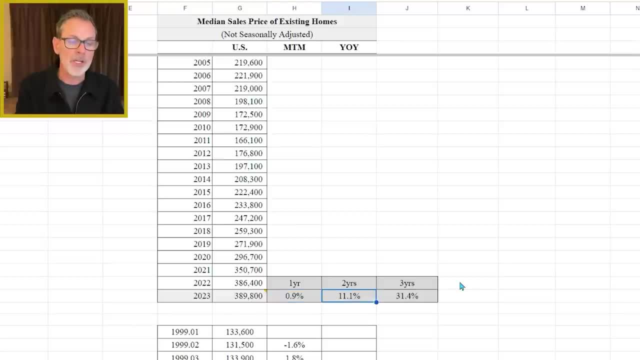 The median sole price of 2012 increased by 5.4%. This short haul is just an estimated 489,000.. a small gain of 0.9% Over the past two years. we saw a gain of 11% and a giant increase of 31.4% over the past three years. going from just under $300,000 in 2020, now it's at more or less 390,000.. Let's also look at prices this last December. So last December last year, it was at $382,600 for the nation as a whole. 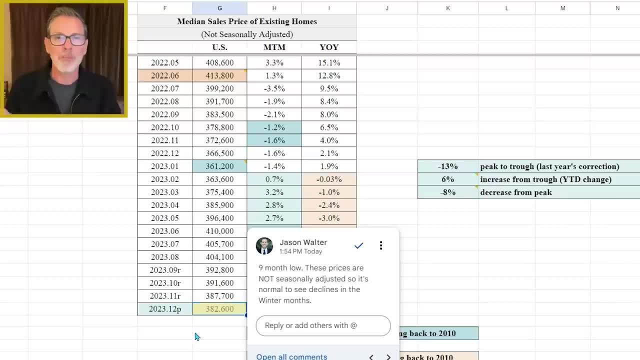 That actually marked a nine-month low in the median sold price nationwide. The last time prices were that low was back in March of 2023. So these prices, keep in mind, are not seasonally adjusted. therefore, it's normal to see prices decrease. 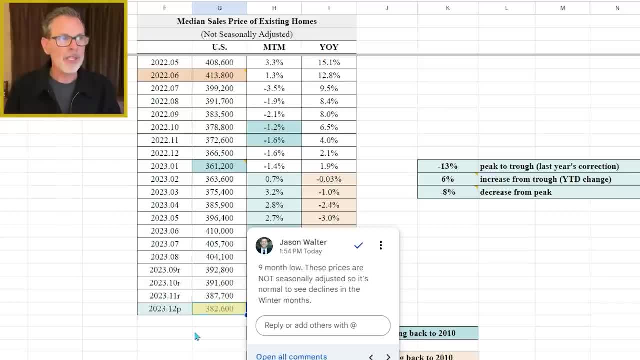 in the winter months. So I would kind of call this a decline in prices due to seasonality. But I also want to share this with you guys as well, because prices decreased by 1.3% on a month-to-month basis, And now prices have decreased for six consecutive months. 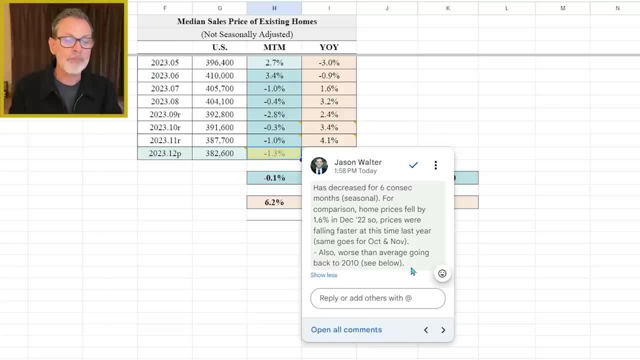 which again is seasonal. For comparison's sake, though, home prices fell by 1.6% in December of 2022. Whereas this December- I should say last December, December 2023, prices decreased by 1.3%. 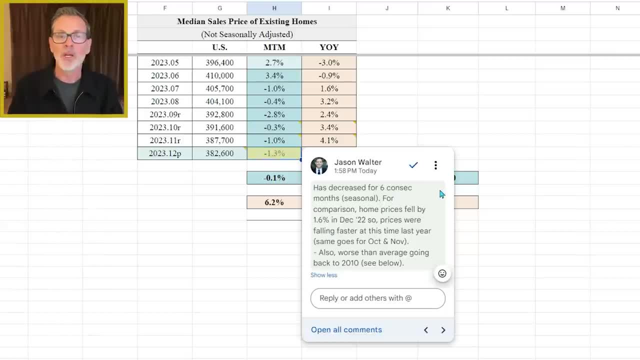 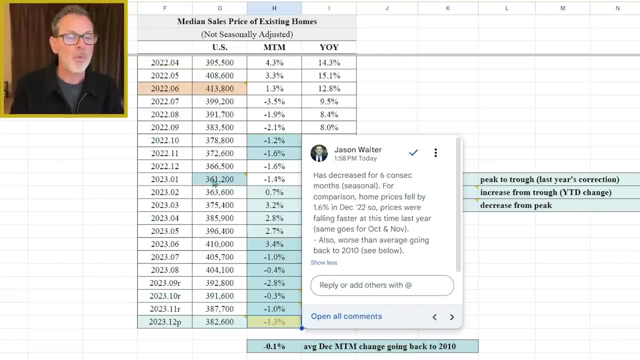 Therefore, prices were falling faster at this time in 2022, compared to this time in 2023.. The same goes for October and November as well. So, for example, this December down by 1.3%, whereas last December or the previous December. 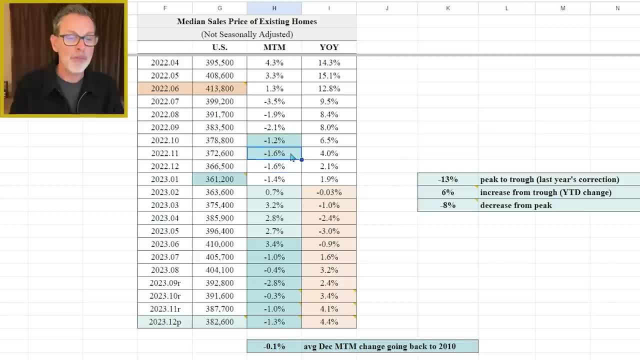 it decreased by 1.6%. In November 2022, compared to October 2022, it decreased by 1.6%, Whereas November 2023, month to month, it only decreased by 1%. Also, in October 2022, it decreased by 1.2%. 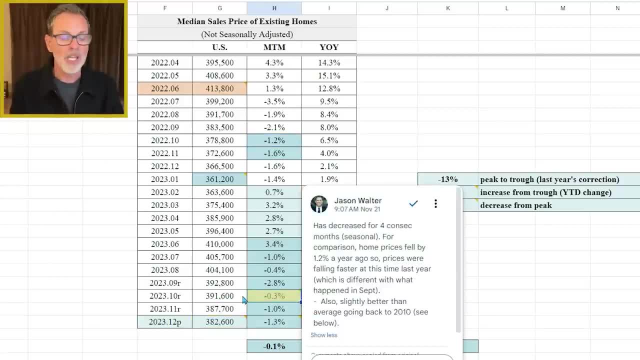 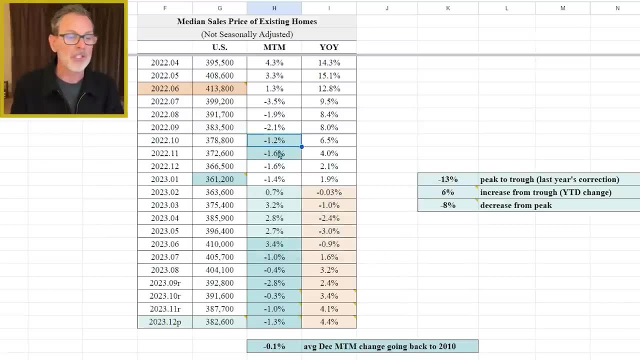 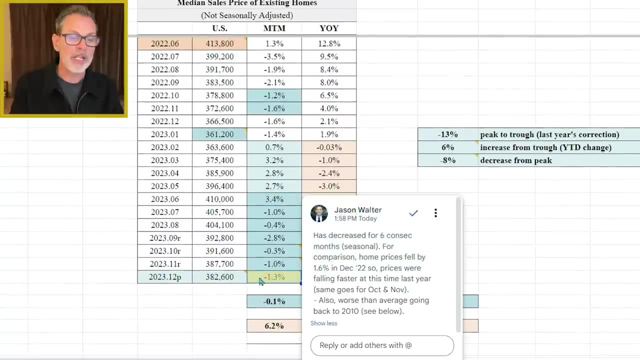 whereas October 2023, it only fell by 0.3%. So, as you guys can see here, the market was falling faster in the last half of 2022 compared and last half of 2023.. One thing, though, that is different though here is that this decline on a month-to-month basis down. 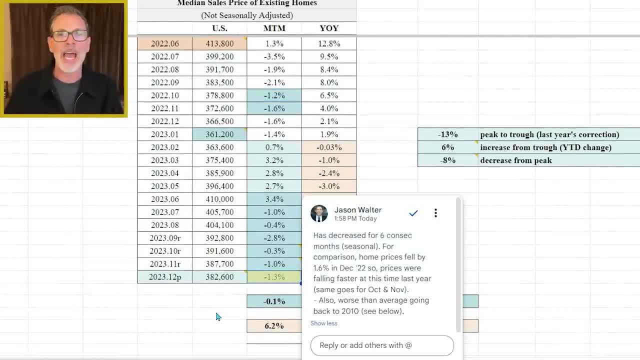 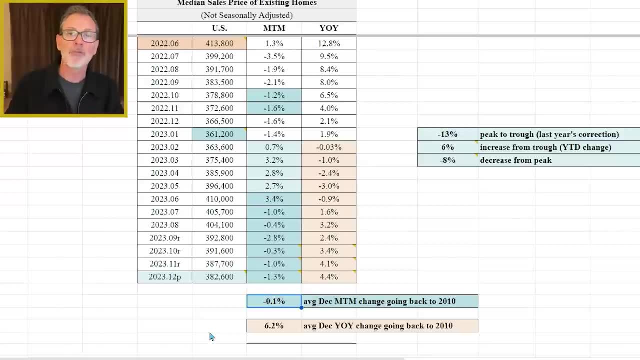 by 1.3% is worse than the average going back to 2010.. So, for example, the average December- this is the average change from November to December each and every year going back to 2010- is a decline of 0.1%, whereas this year it decreased by 1.3%. All right, that was the. 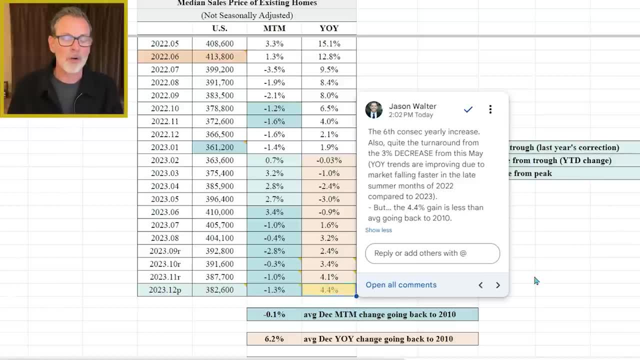 month-to-month changes. Let's have a look at the yearly changes here, or the year-over-year changes, because this December it increased by 4.4% compared to December 2022. That marked the sixth consecutive yearly increase. Also, this is quite the turnaround because back in May, 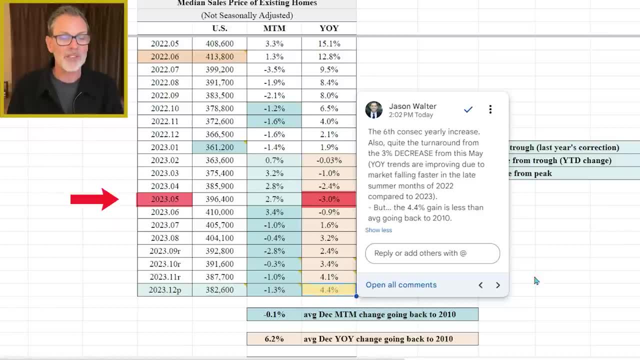 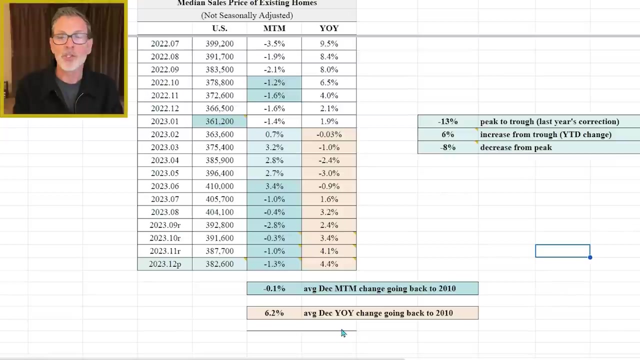 of 2023, home sold prices decreased by 3%, So therefore the year-over-year trends are improving, due to the market falling faster in 2022 compared to 2023.. However, though, the gain of 4.4% year over year is actually much worse than the average going back to 2010, because the average is a gain of 6.2%, quite a bit higher than the 4.4% we saw this December. But wait, there's more, because I also want to share how the prices, or how home prices, have changed over the past several years here. So over the past two years- this is December of 2021, when prices were at $359,000. 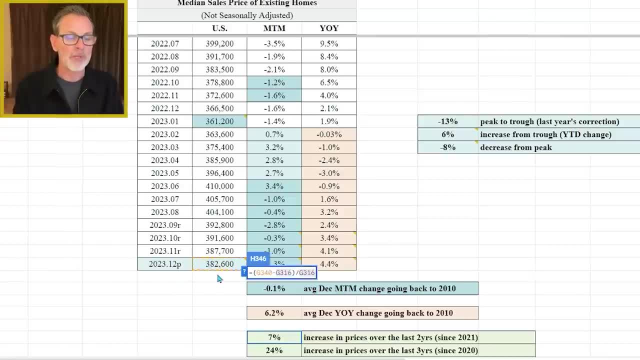 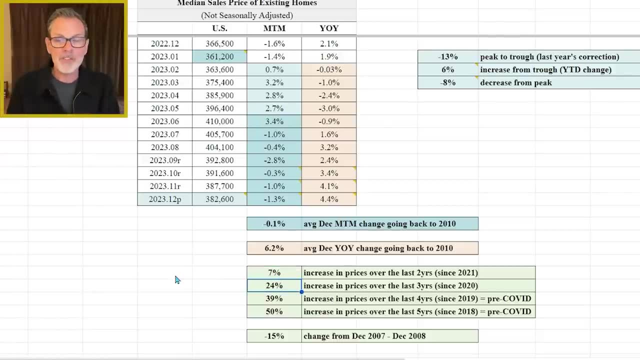 more or less. now it's at $382,000 approximately. That's a gain of 7% over the past two years. Over the past three years, since December of 2020, prices have surged by 24%, Also a giant increase of 39% since December of 2019,. 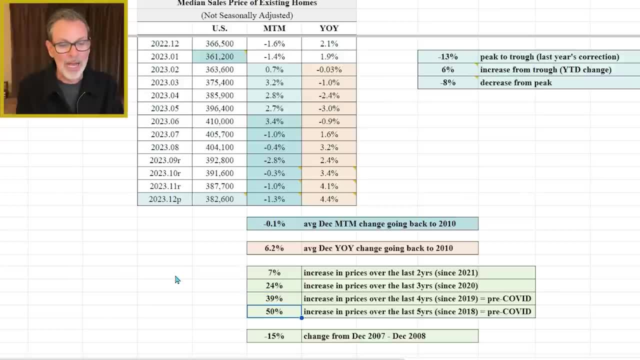 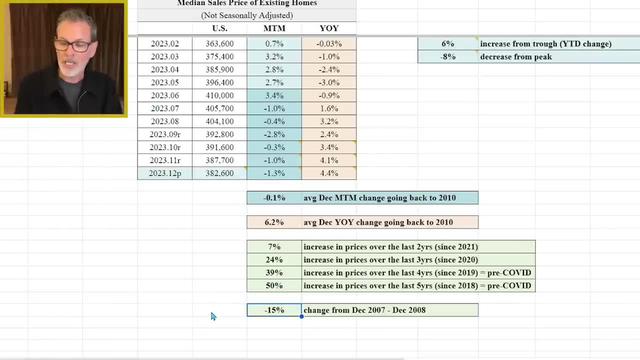 and also a giant increase of 50% over the past five years. Also, if you guys are looking for a housing market crash, if you guys think we're going to see a housing market be in worse off or worse off than 2008,, here's what happened in December of 2007 through December of 2008,. a giant decrease of 15%, whereas this last December an increase of 4.4%. Okay, let's change gears slightly here and talk about inventory levels here. So on a national level, total house inventory by the end of December was at 1 million units, down 11.5%. 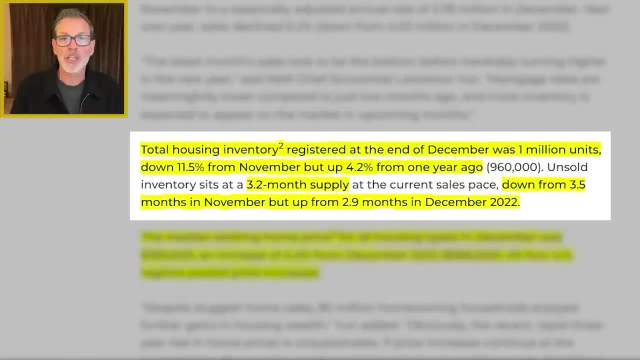 from November, but down 4.2% from one year ago. That 1 million units, I believe, includes some pending home sales, because that figure there is much higher compared to realtorcom as well as altosresearchcom. In any case, though, we're still down by 4.2%. from 12 months ago. Also, the month supply in December was only at 3.2 months. That was down from 3.5 months we saw back in November and up, though, compared to the 2.9 months we saw. 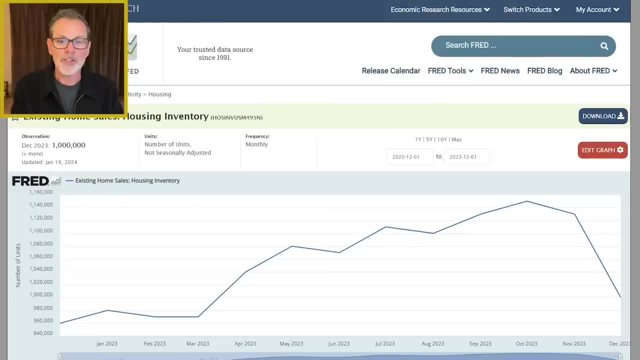 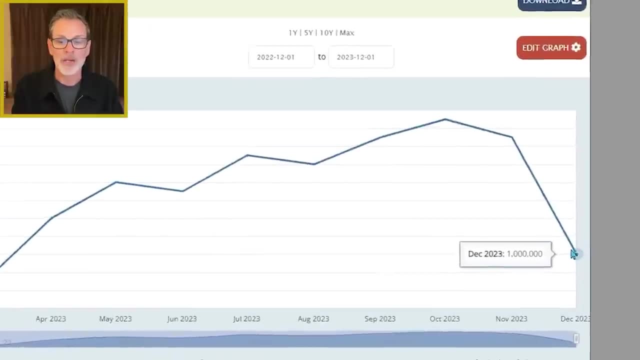 back in December of 2022.. So in regards to that, here's a good Uncle Fred here looking at inventory levels over the past 12 months. So right now it's at 1 million, down greatly from the 1.15 million we saw back in. October of 2023.. But at 1 million units, it's still above the 960,000 we saw 12 months ago. Also, regarding the month supply at 3.2 months, this is down from the peak at 3.6 months. 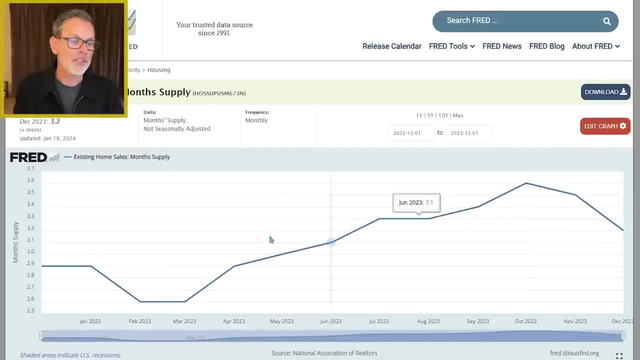 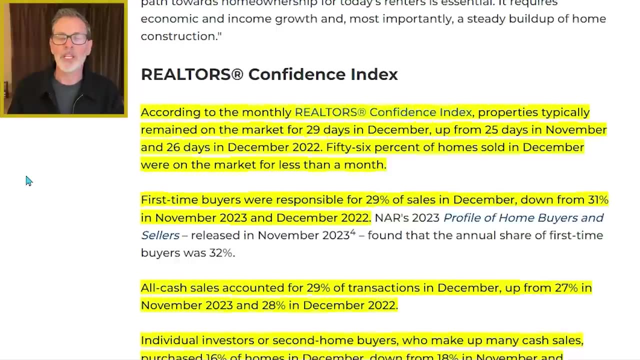 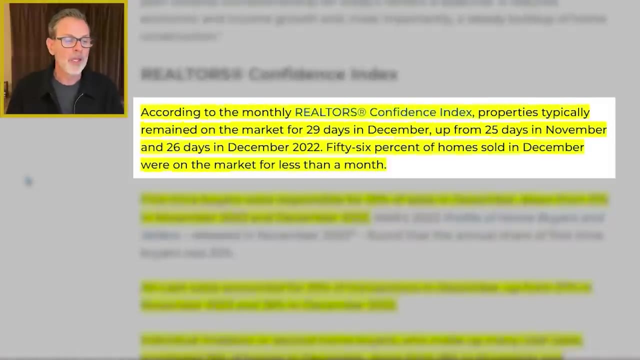 back in October, But at 3.2 months. this is still higher compared to 12 months ago at 2.9 months. Also based on their monthly survey, here, days in the market was at 29 days in December. That was up from 25 days in November and also a little bit higher compared to the previous. 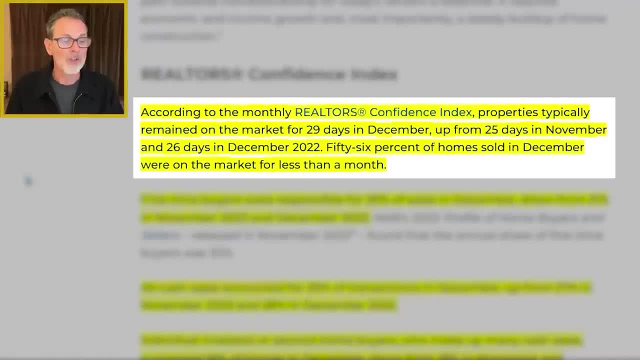 market. So we're looking at a little bit higher than the previous market. So we're looking at a little bit higher than the previous market. So we're looking at a little bit higher than the year, at 26 days. Also, 56% of houses that sold in December were on the market for less than one.